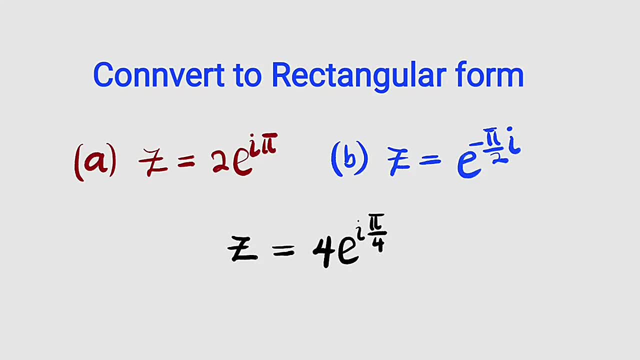 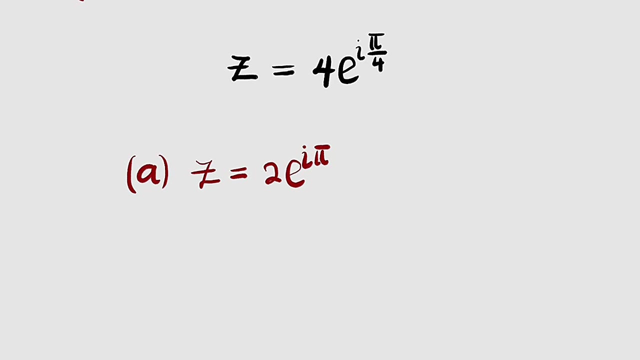 Hello, good day viewers. In this tutorial we are going to learn how to convert a complex number from its exponential form to rectangular form, and we have only three examples, and all other problems remain the same. The first question: we are given a complex number equal to 2e to the i pi. Remember if you have a 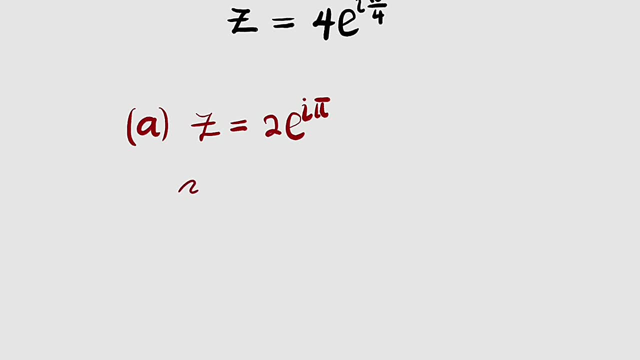 complex number like this rectangular form is equal to z, equal to a plus bi, and hence this complex number can easily be converted into this form, because if you have r e to the i theta, it is the same thing as r multiplied by cosine of theta plus i sine of theta. and from here we can. 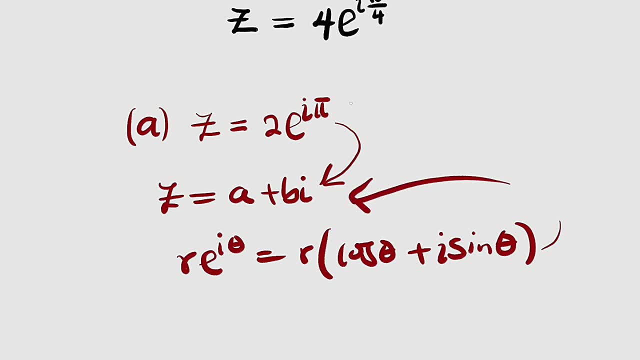 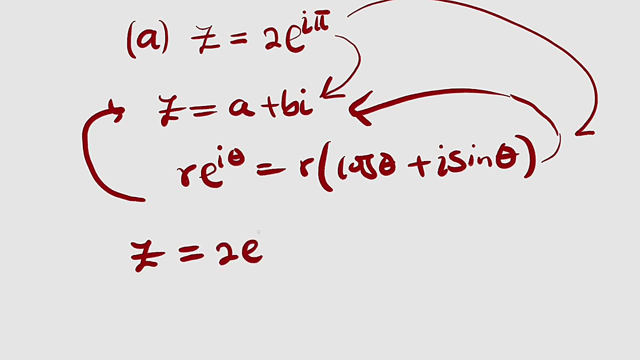 take it back to the rectangular form. This means that we have to take this one into its polar form, then take it back to rectangular form, and that's what we are going to do in this tutorial. So, therefore, if you have z equal to 2e, to 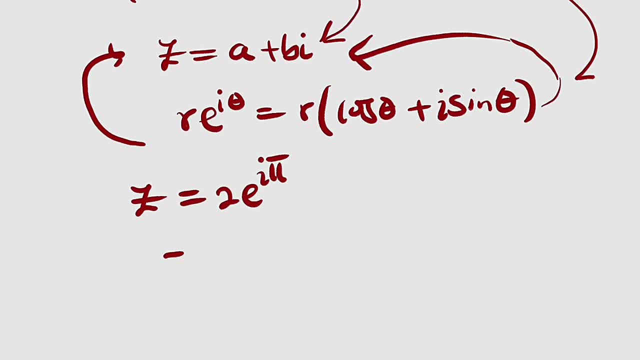 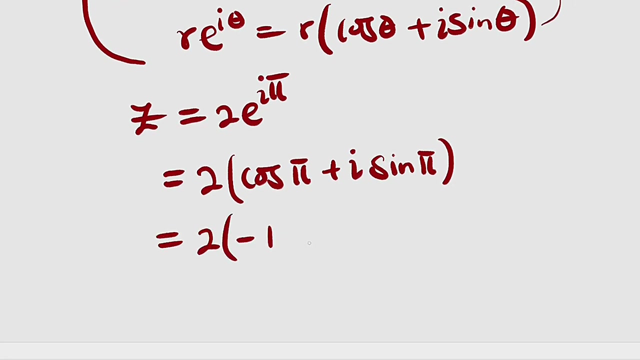 the i pi. this is the same thing as 2 multiplied by cosine of pi. then plus i sine of theta Sine of Pi. Cosine of Pi is equal to negative one. therefore, this is equal to two multiplied by negative 1 plus i multiplied by sine of Pi. What is sine of? 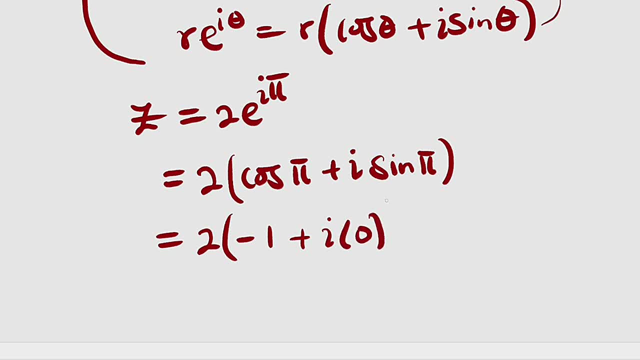 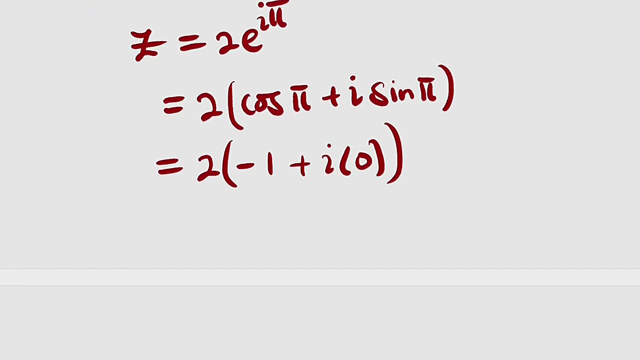 Pi is equal to zero, right, And i times zero is equal to zero. so if we expand, you only have to multiply by negative 1, which is equal to. Therefore, this complex number is nothing but negative 2.. Now let us take the second one. 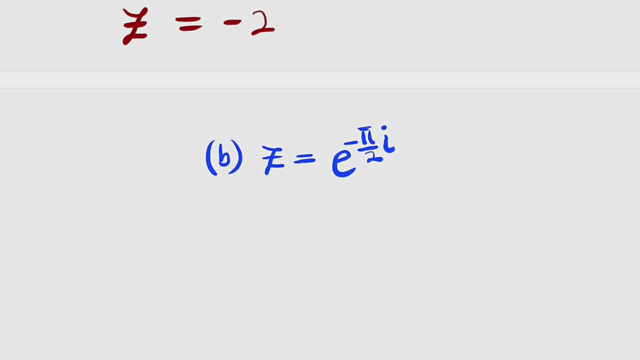 Here is the second one. We are given a complex number equal to e, to the negative pi divided by 2i. So first of all let us convert it into its polar form. So we have z equal to r, The coefficient here is the r, but here we have 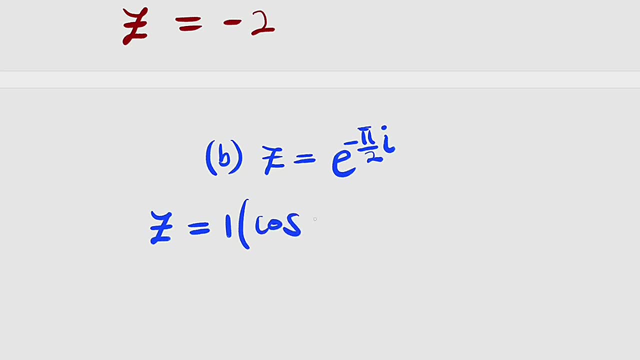 only 1.. Then inside we have cosine of what Negative pi divided by 2 plus i sine of negative pi divided by 2.. Now let us simplify what is under the parenthesis. z is equal to 1 times whatever, It is the same thing. We have cosine of negative pi divided. 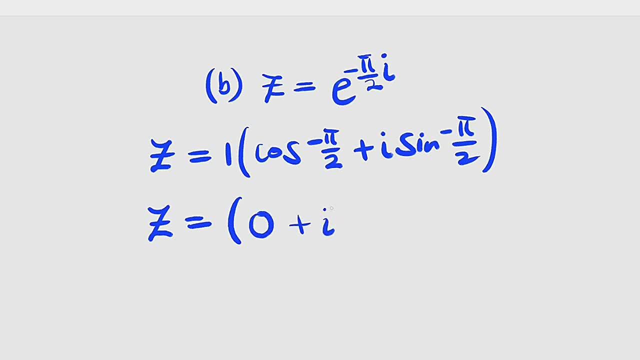 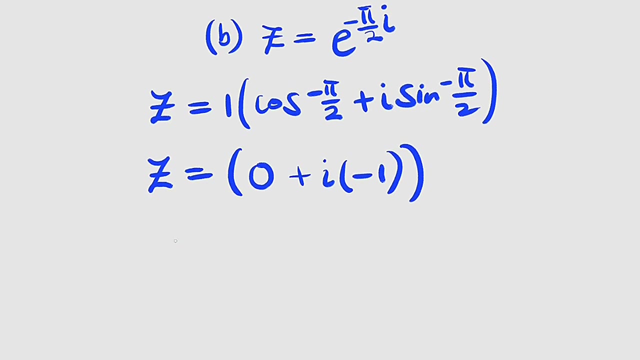 by 2, which is 0 plus i. multiplied by sine of negative pi, divided by 2 is negative 1.. So the only 2 we have here is what i times negative 1, which is negative i plus 0 is still negative i. Therefore. 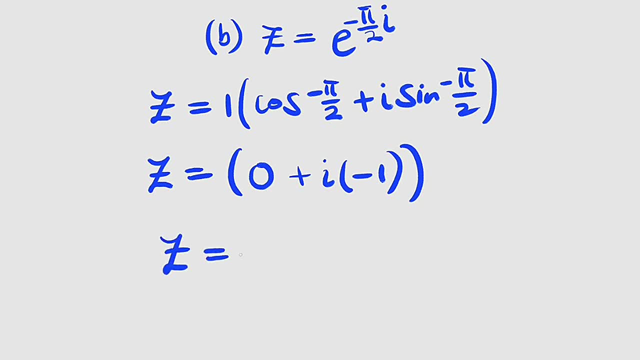 this complex number in its rectangular form is just negative. i Let us take the last one, The last one. we have a complex number equal to 4e, to the i pi divided by 4.. First of all, we are going to transform it into its polar form. 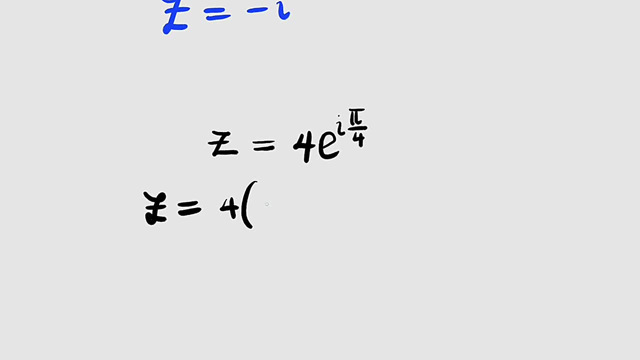 z will be equal to r, which is 4 multiplied by cosine of pi divided by 4, plus i sine of what pi divided by 4.. And what is cosine of pi divided by 4 is root 2 divided by 2.. Likewise, 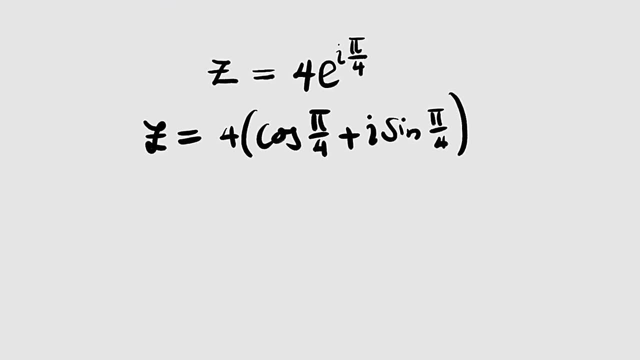 sine of pi divided by 4 is root 2 divided by 2.. So this is equal to 4 multiplied by root 2 divided by 2, plus i root 2 divided by 2.. If we distribute, you will have 4 multiplied by root 2 divided. 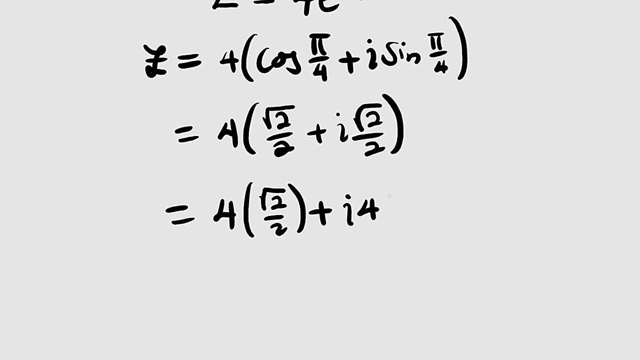 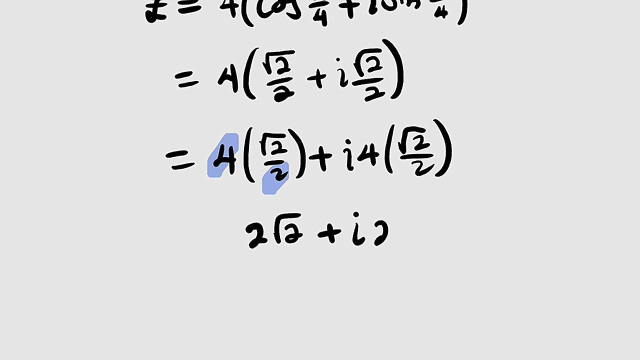 by 2 plus i, 4 multiplied by root 2 divided by 2.. From here you can see: 2 will go into 4 two times. So what do we have? We only have 2 root 2 here, plus i, multiplied by 2, root 2, which we can. 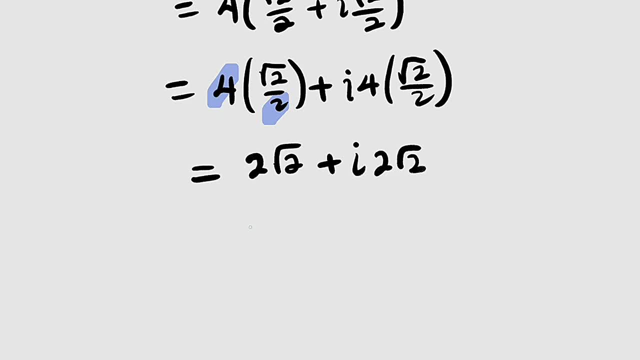 rearrange as what: 2 root 2 i. So this is 2 root 2 plus 2 root 2 i, And hence this is our rectangular form of our complex number. So let me give you one to try, because this is: